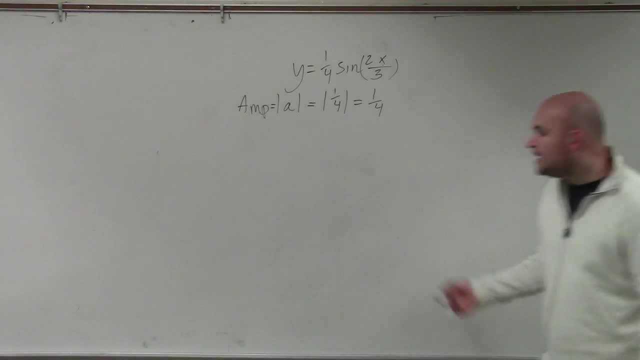 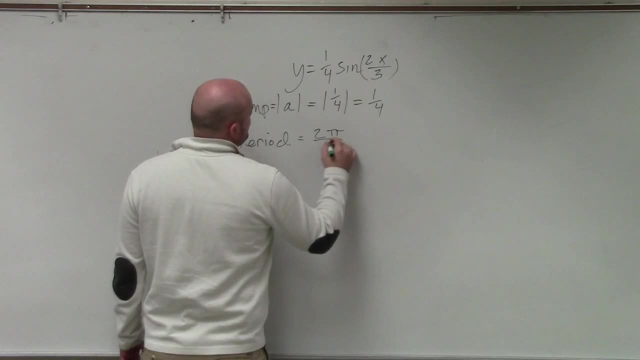 if it's negative, it's going to be positive. If it's positive, it's going to be positive. The period is going to be 2 pi divided by b. Now, this one can bring in some problems, because we need to. 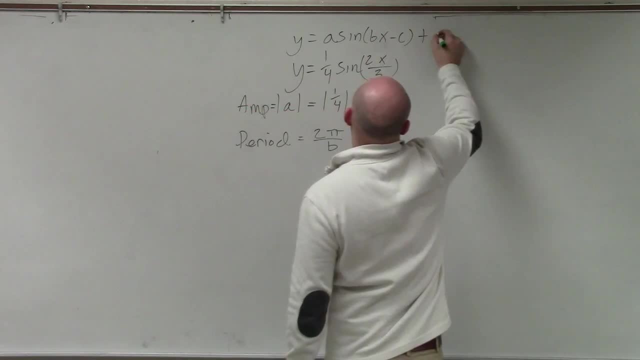 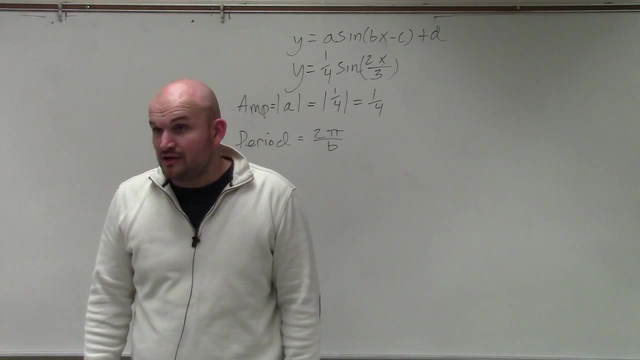 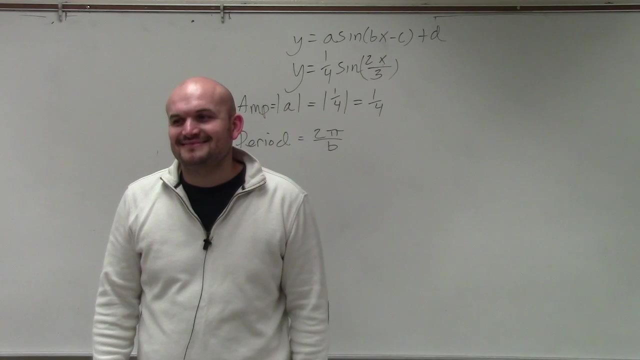 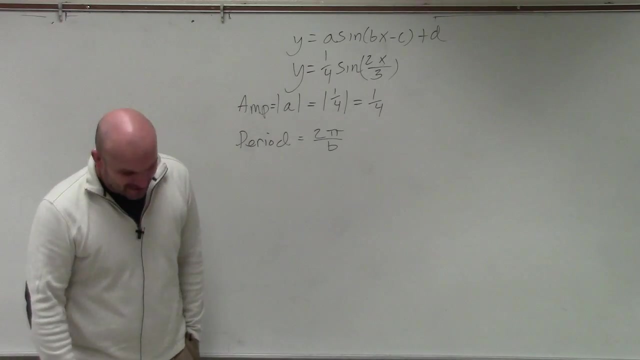 So remember, first of all, where is b and how does b relate to in this problem? b is the coefficient of our input value. Yes, So what we need to do is identify the coefficient of our input value. okay, The? 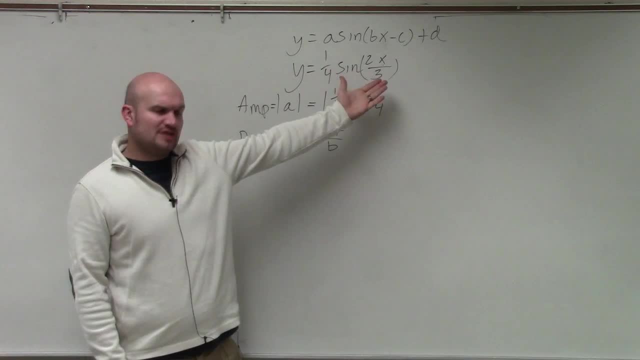 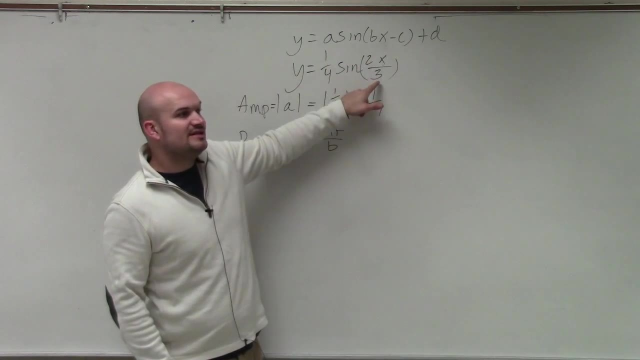 coefficient of our input value. a lot of you guys might say: well, it's 2, which, yes, 2 is being multiplied by x. However, we also need to understand that yes, 2 is being multiplied by x, but 2 is also being divided by 3.. So we just need to understand that yes, 2x divided. 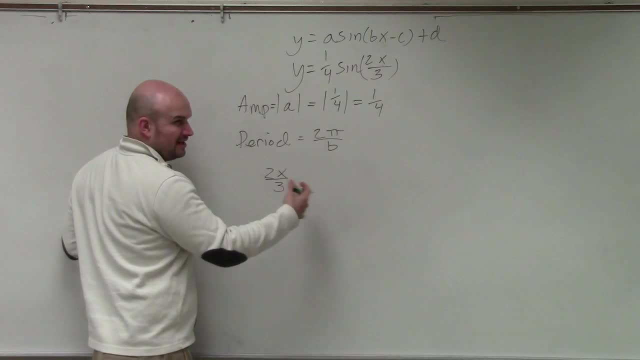 by 3, when we're writing like angles. a lot of times you know we wrote that especially like 2 pi over 4 and so forth. But in the terms of this, when we're trying to find the 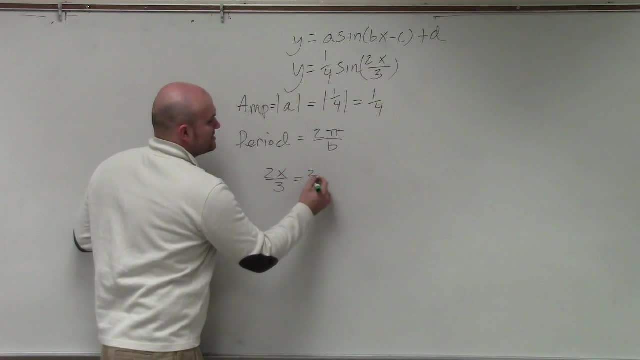 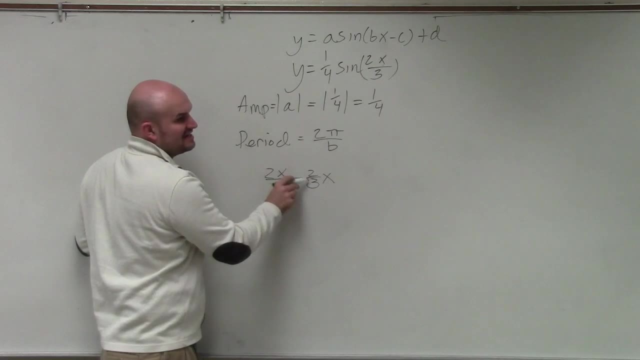 coefficient. just understand that 2x divided by 3 is the same thing as 2 thirds times 2 times x. Do you guys agree with me? But if I put it in this way, we can see that b is actually 2 thirds, not 2, because it is 2, but 2 is divided by 3.. So therefore I have 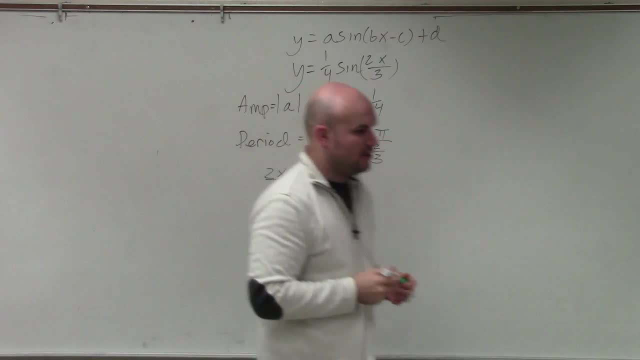 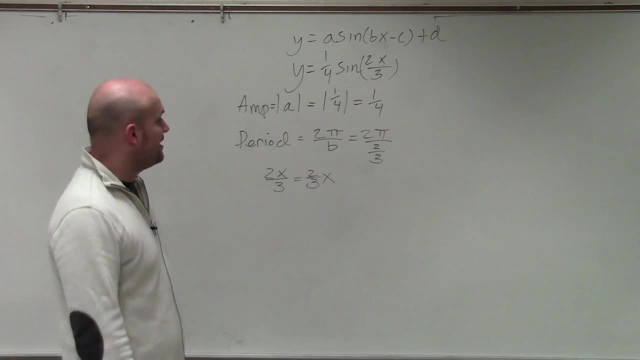 2 pi divided by 2 thirds. And I have a lifelong goal of having students that whenever they see fractions, not freaking out and understanding, oh wow. I always said Mr McLogan and he always said: whenever you're dividing by a fraction, you'll have division of fractions. 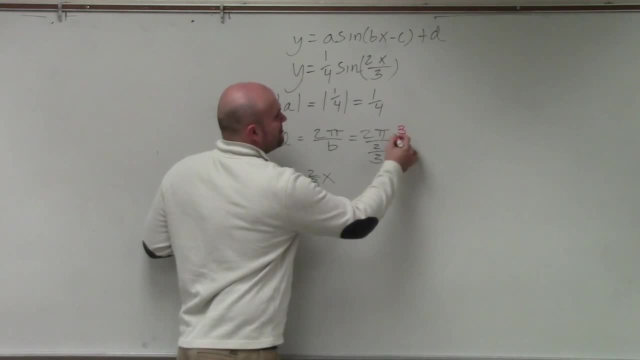 you just need to get the fraction off the denominator By multiplying by the reciprocal 2 thirds times 3, halves is just going to be 1.. Now I have 2 pi times 3 over 2. Those divide out and I'm left with 3 pi.